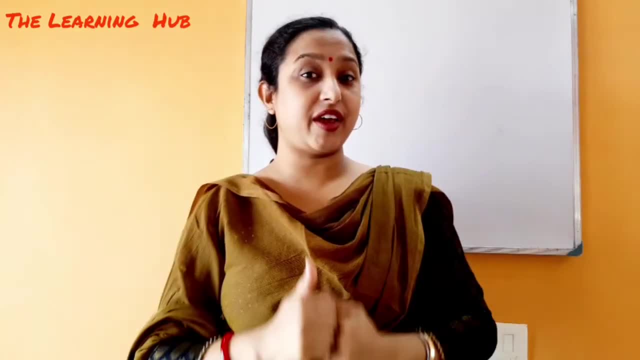 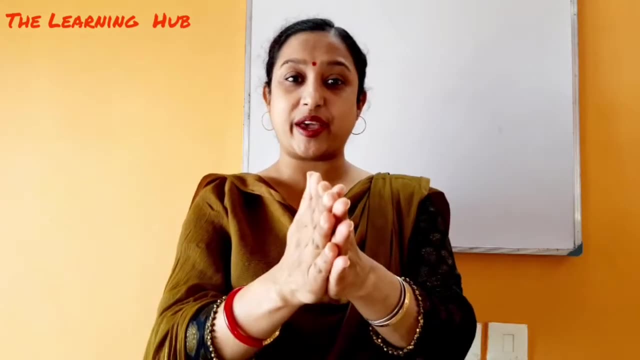 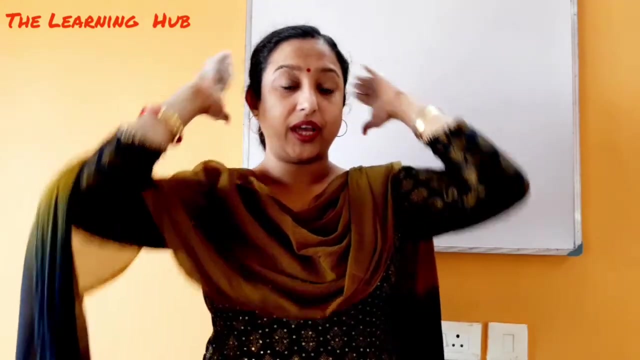 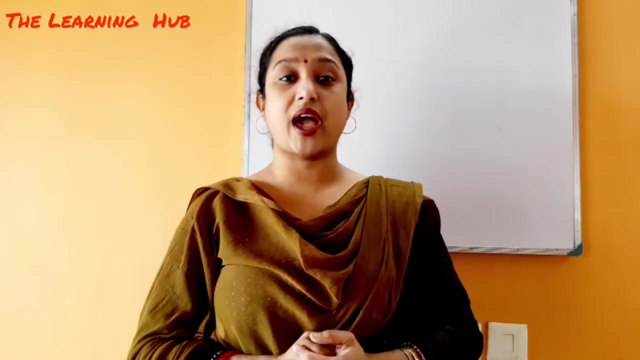 Five. Very good, Well played Now a little bit faster. One, two, three, four, five. Then one, two, three, four, five, Very good. Now we will do another movement: Snap your fingers two times and shake your hands two times. 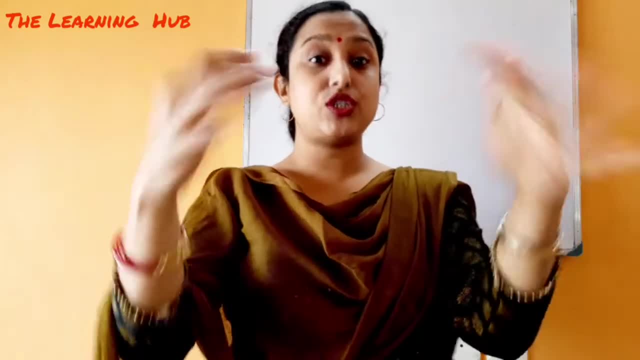 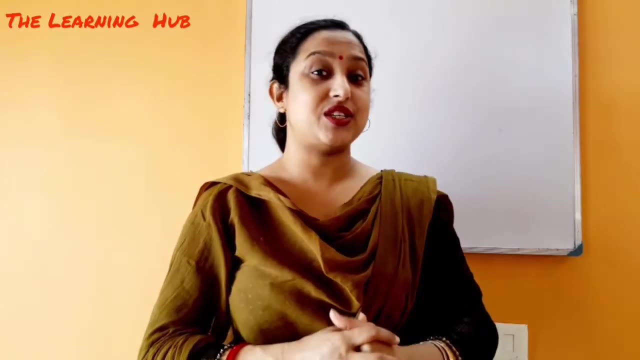 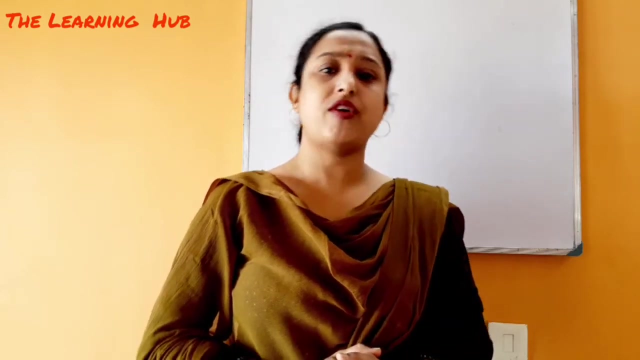 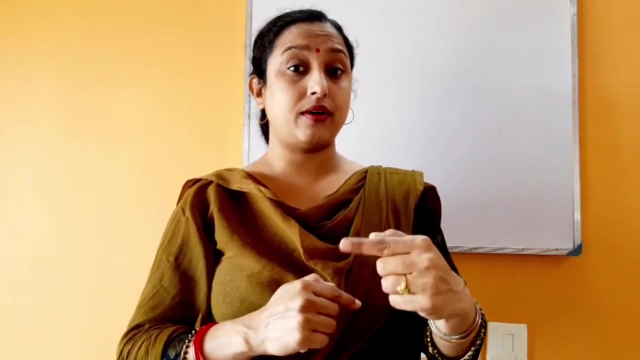 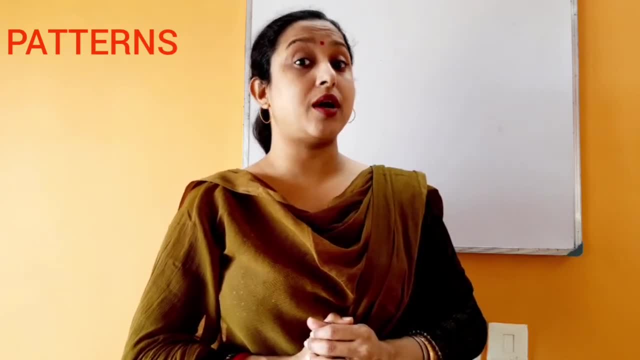 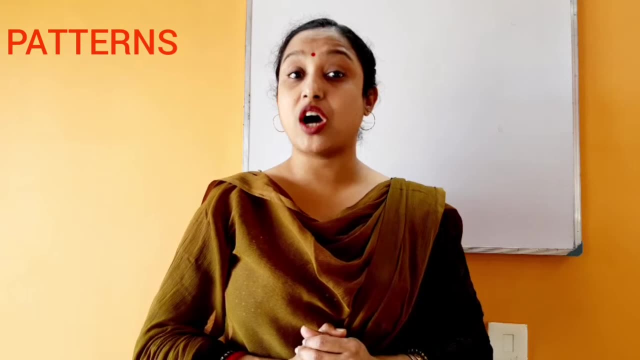 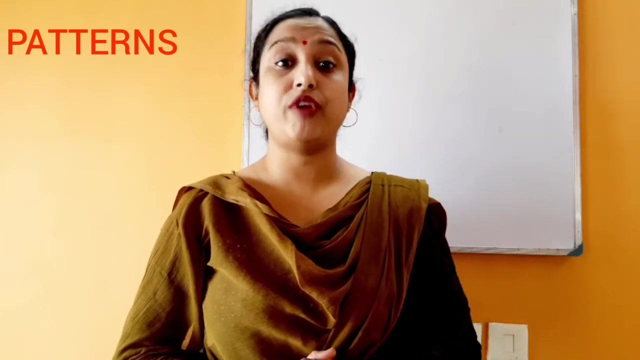 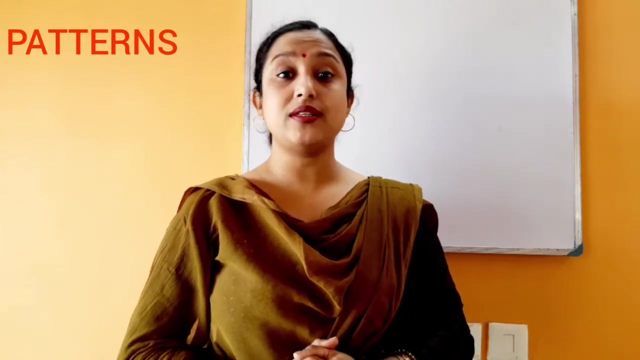 And in this game we have observed A particular pattern Right. So, children, today we are going to learn pattern What Pattern? But what is pattern? Pattern is a way in which some things are arranged or organized in a particular rhythm or sequence. 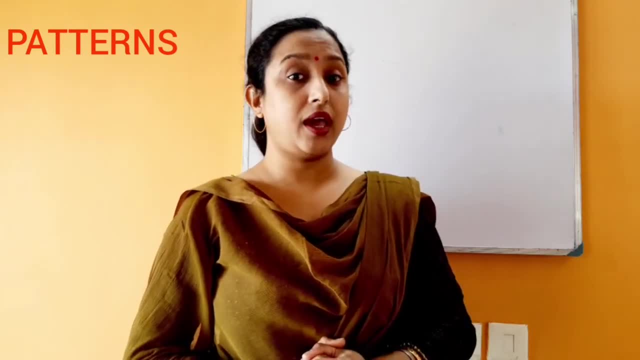 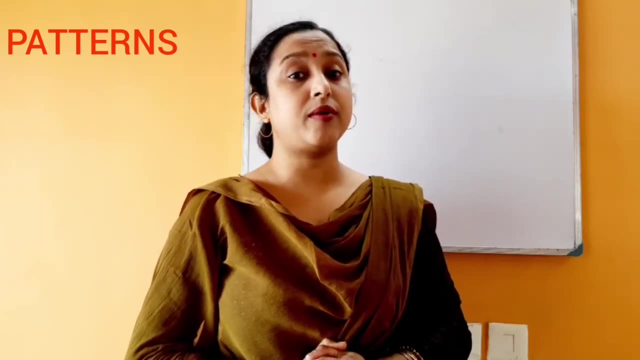 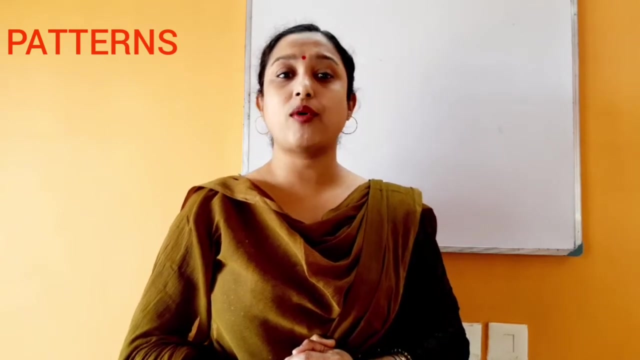 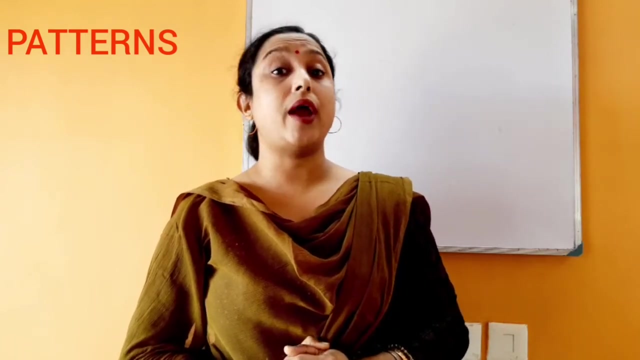 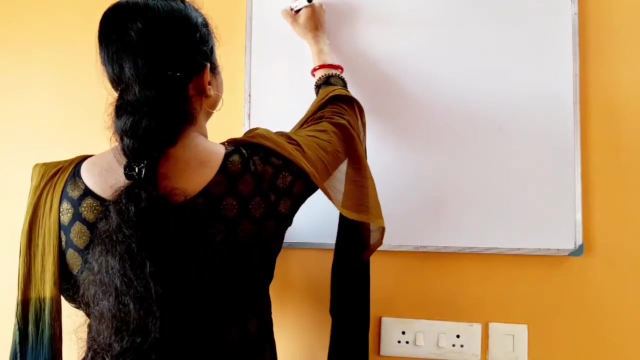 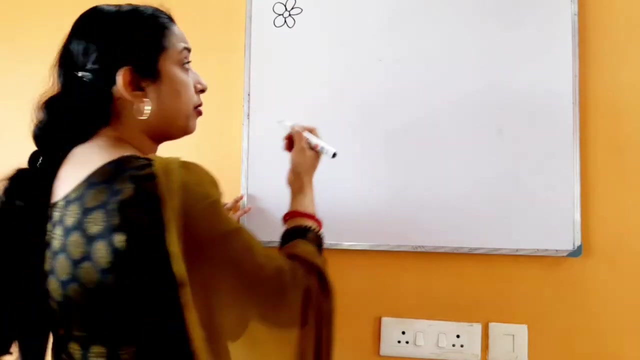 I repeat, Pattern is a way in which some things are organized or arranged in a particular rhythm or sequence. so to clear the concept of pattern now I'm going to give you some examples. so children look at the board, observe very carefully and recognize the pattern. what is this? it's a flirt. next, 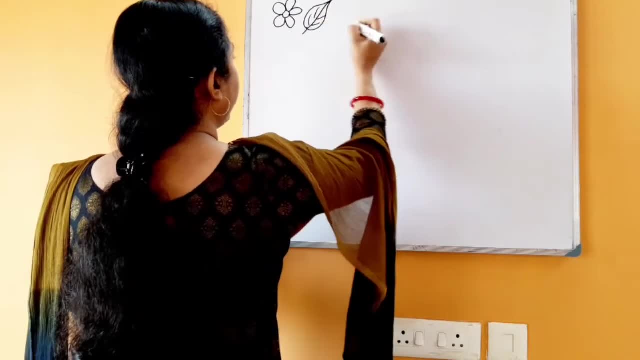 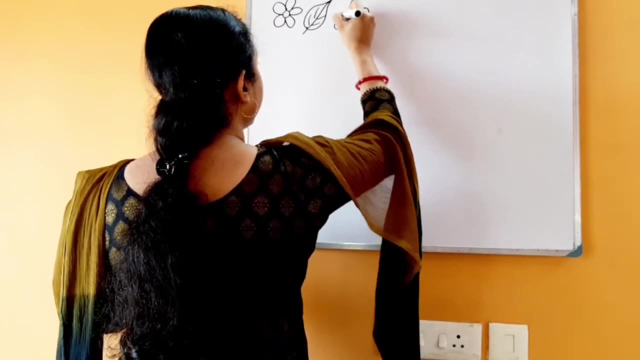 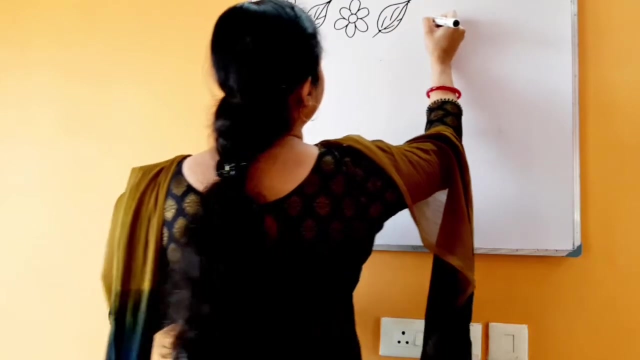 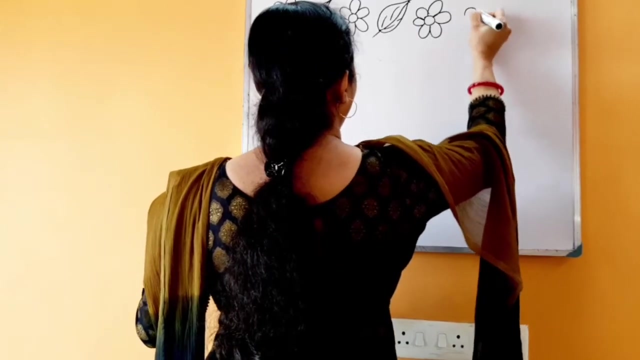 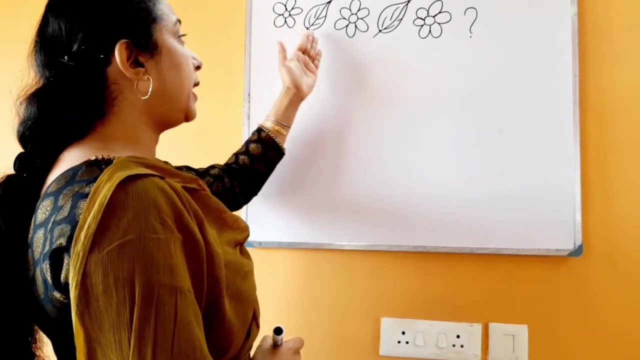 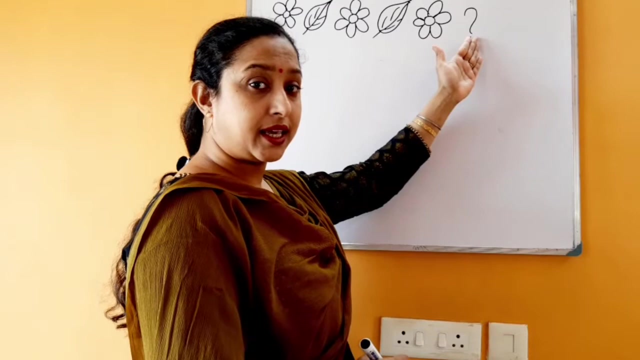 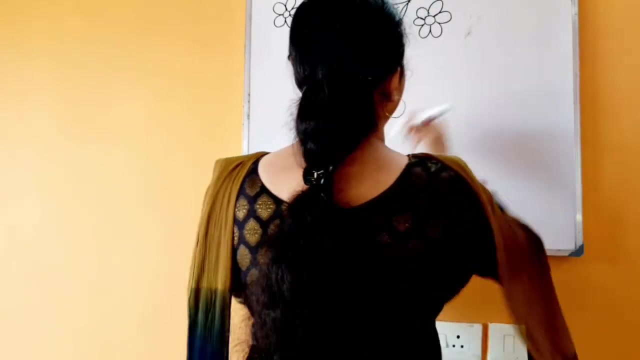 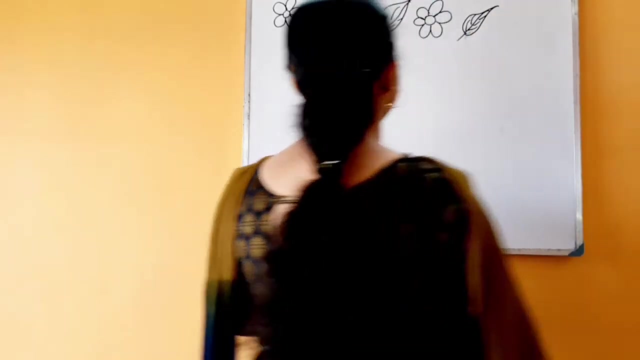 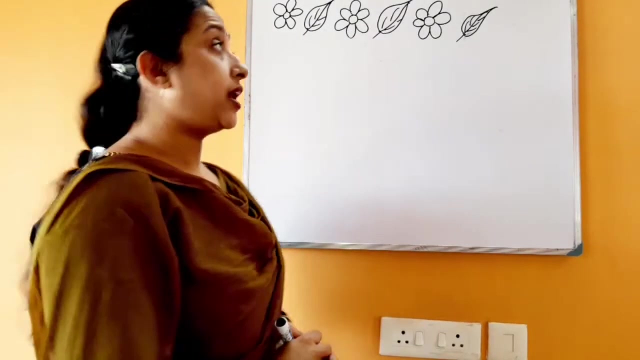 this is flip again a flirt, and again again flower. now, what will come next? observe the pattern very carefully: flower, leave, flower, leave, flower. then what will come next? yes, so you have to raise and then and there is a complete pattern. it's an alternating pattern. here we have arranged objects, alternative boys, one by 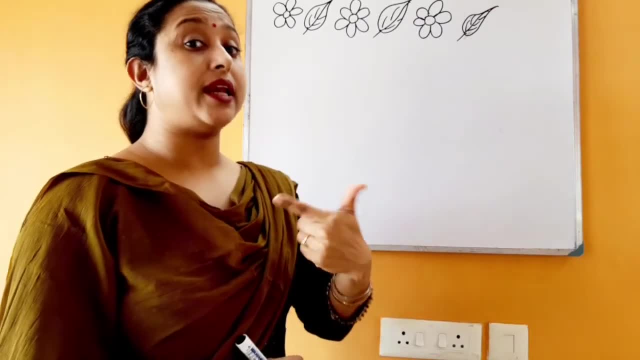 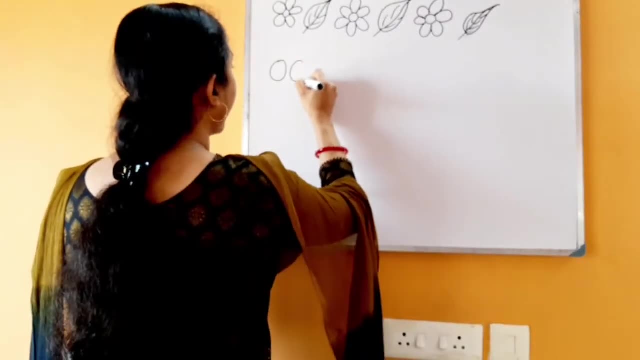 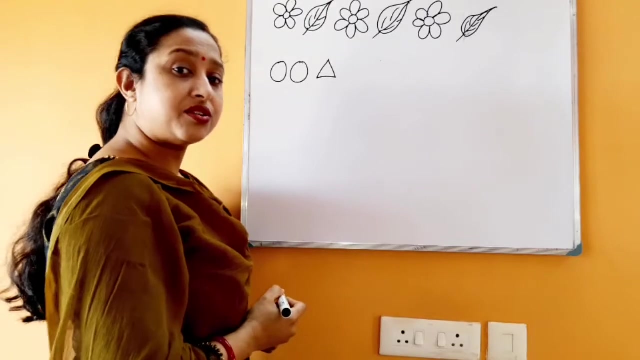 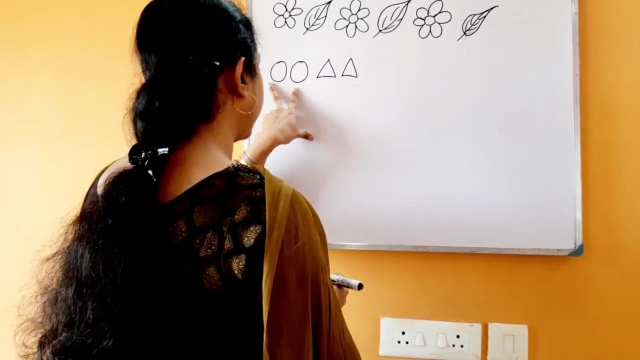 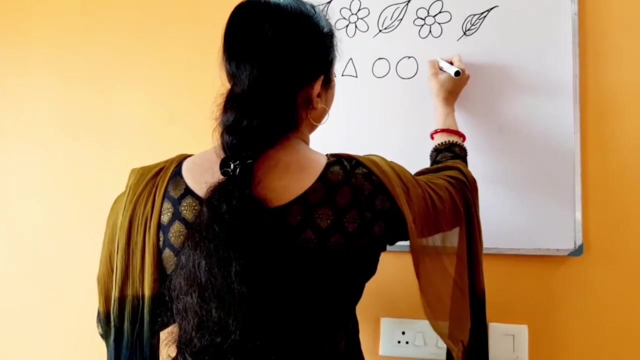 one right now. the next example: Which shape is this Circle? How many circles are there Two? Which shape is this Triangle? How many triangles are there Two? So two circles, two triangles, again two circles. Then what will come next? 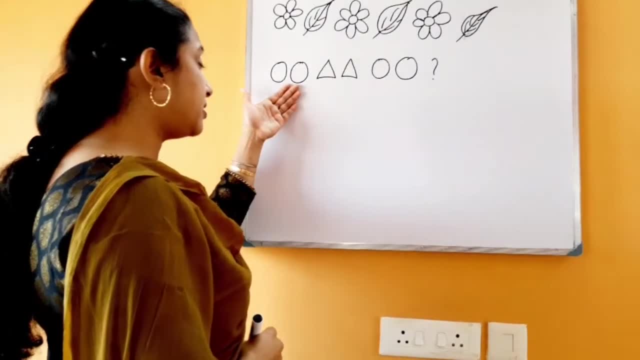 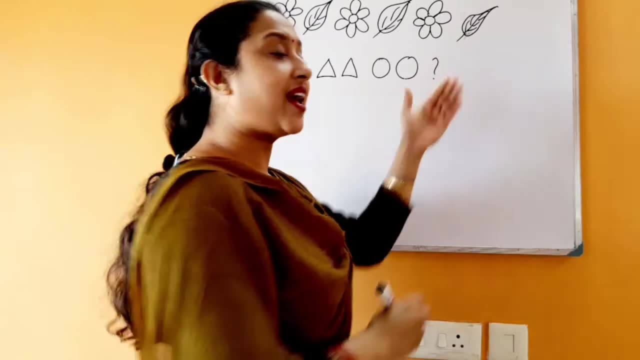 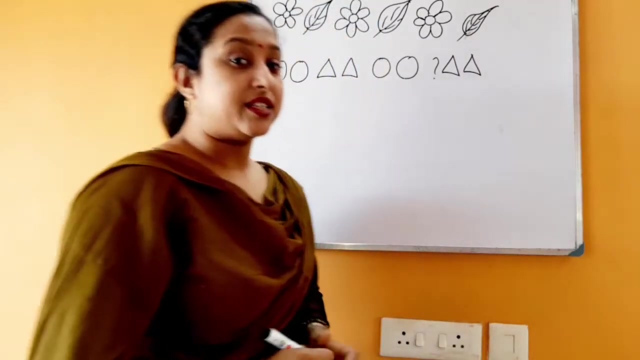 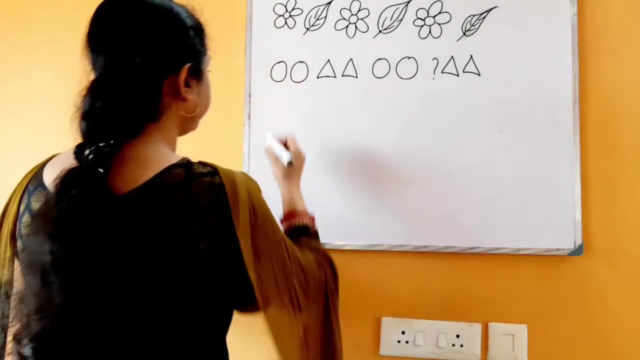 Observe the pattern very carefully: Circles, triangles, circles, then, yes, triangles. So we have to draw triangles over here. Okay so, children, this is also a pattern. Now the next example: Star circle square. 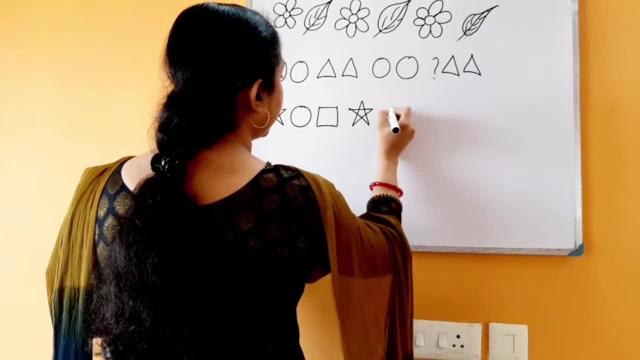 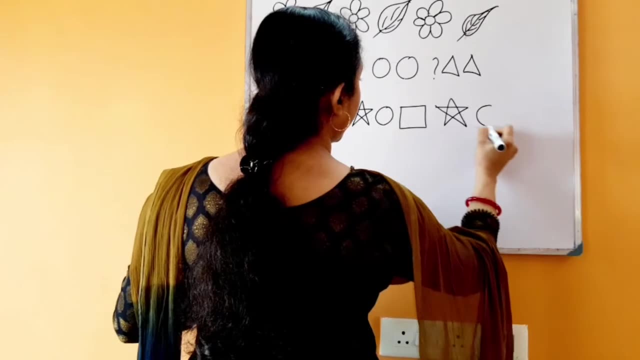 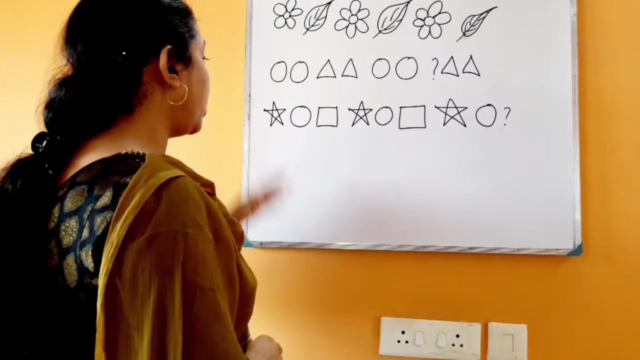 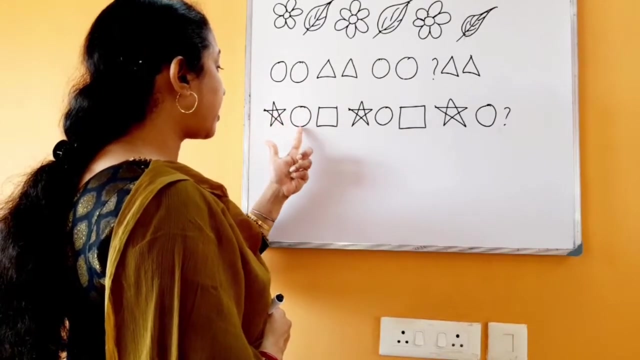 Again, star circle, square, Star circle. then what will come next? Observe the pattern very carefully. You can assume: A, B, C. See, this is star, this is circle and this is square. These are the different shapes. 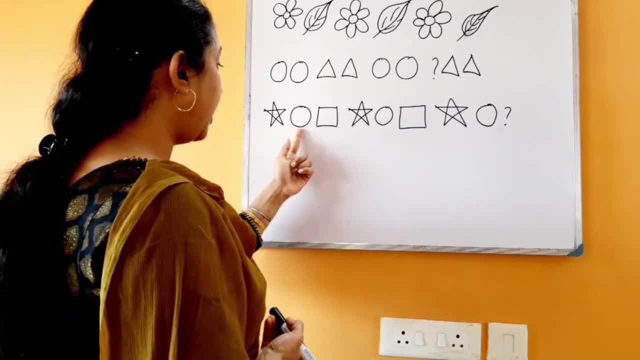 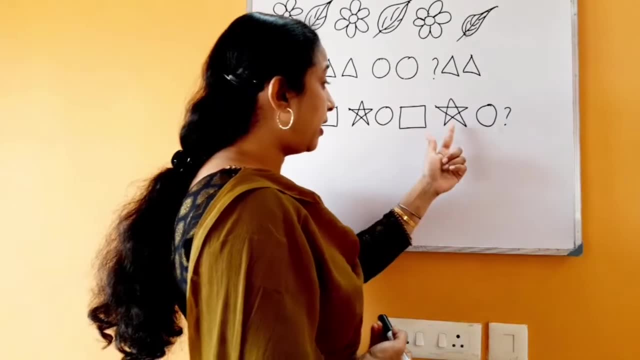 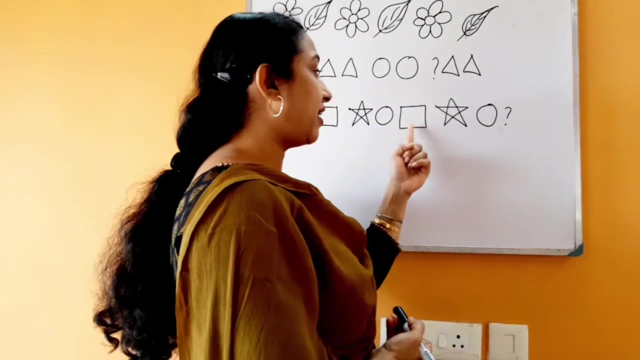 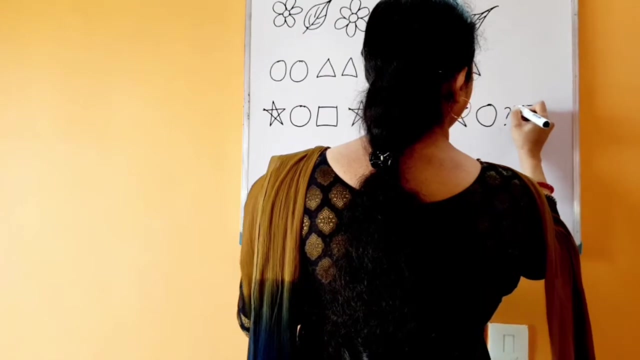 So you can assume A, B, C, Then again A, B, C, Then again A B, then what will come next? Yes, C, C means here the square. So we have to draw a square. then like this: 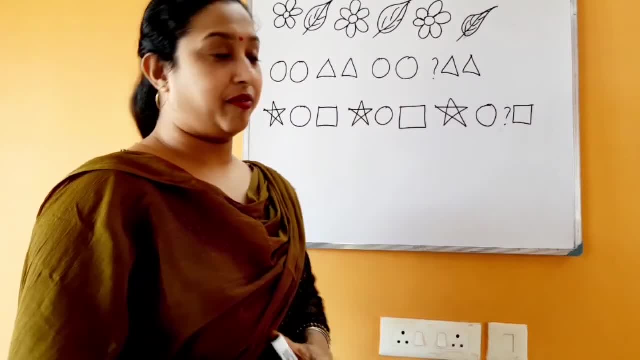 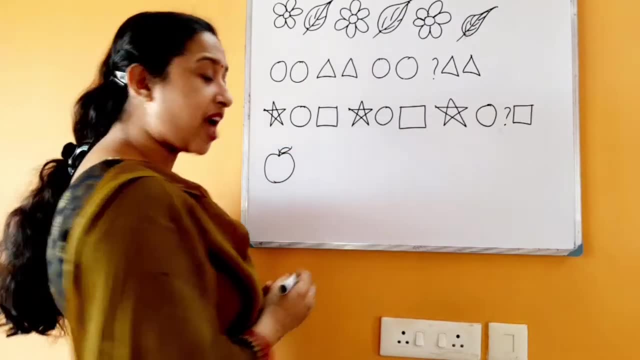 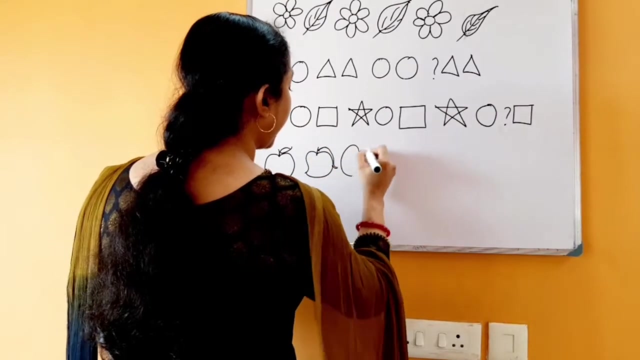 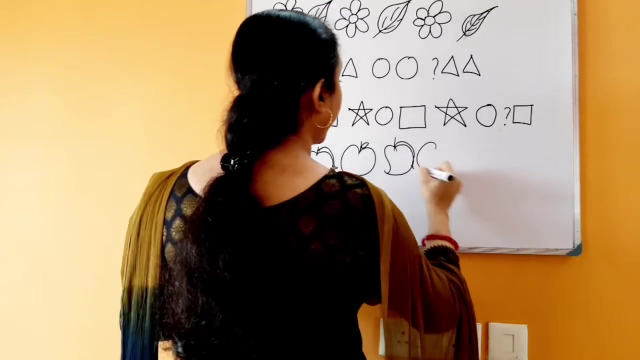 So it's a complete pattern. The next example: what is this? An apple, then mango, again apple, then again mango, then again apple, then again apple. So what will come next? 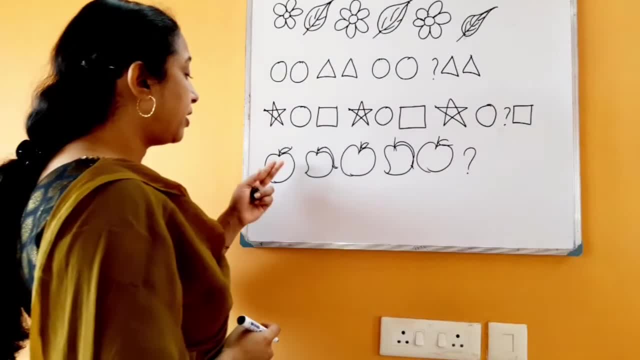 Observe: apple, mango, then again apple, then again mango, then again apple, then apple, Then, yes, mango. So let's complete the pattern. The next example: what will come next? 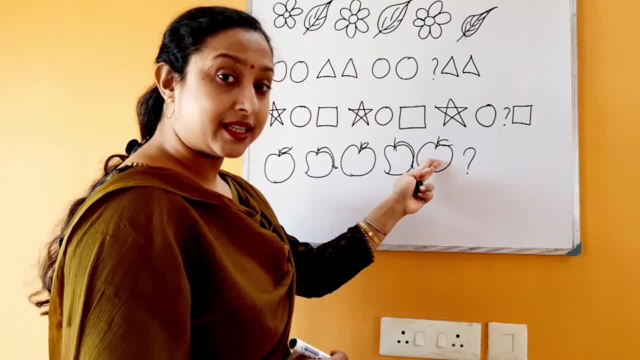 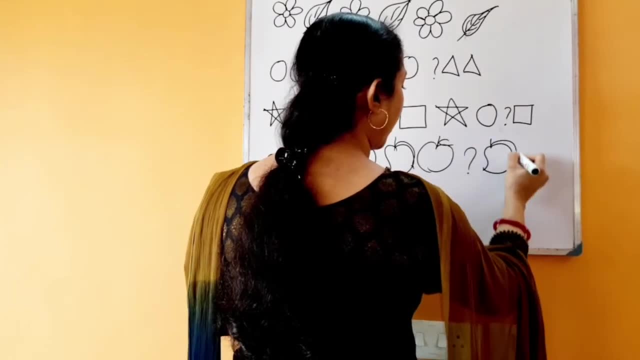 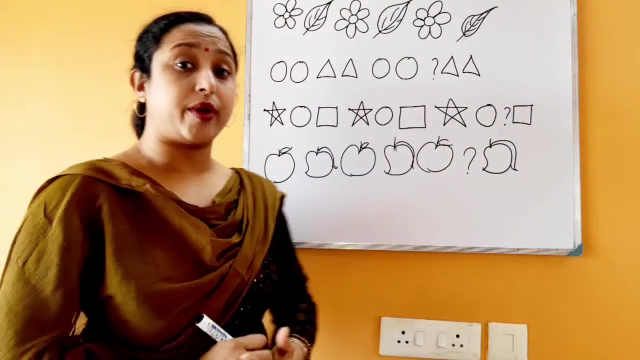 Then, yes, it's a complete pattern: Apple, Mango, Apple. Then, yes, mango. So let's complete the pattern: mango. So, children, we can see that different types of objects are arranged in a particular rhythm or sequence. 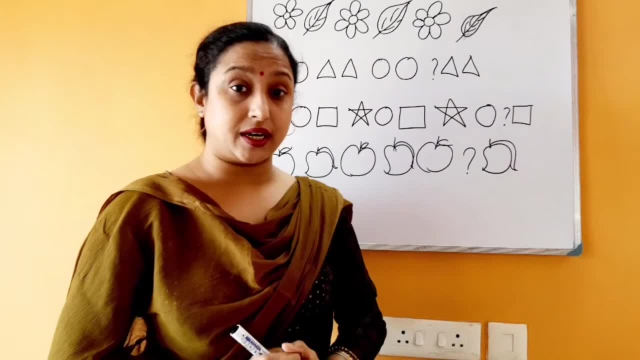 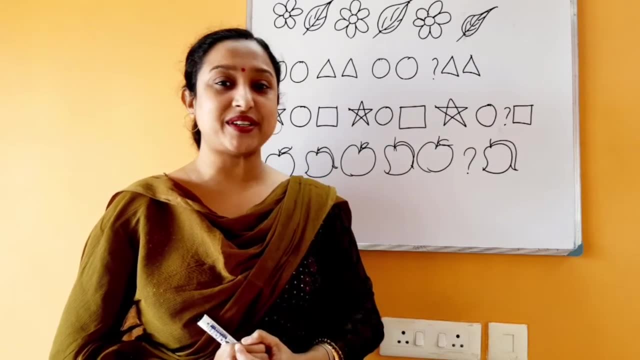 So these are called patterns, Right? So now we have to draw a circle, then again apple, then again apple, then again apple, Apple, Right. So now it's time to do an activity, So let's enjoy the activity. 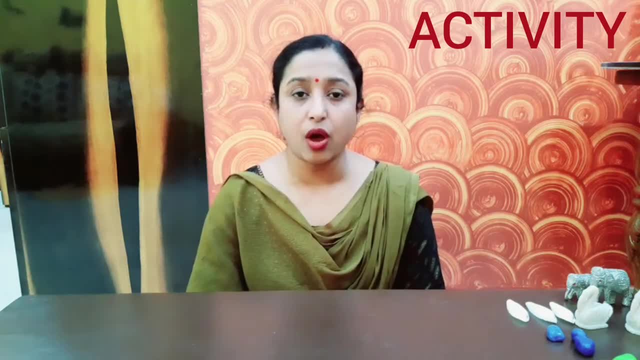 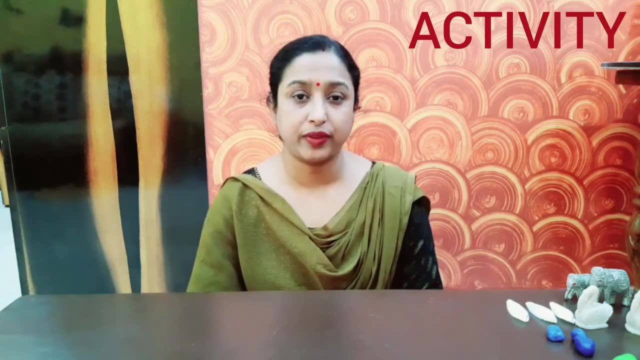 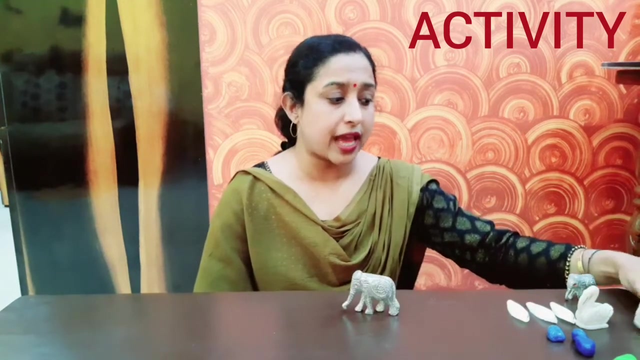 So, children, we can see patterns all around us: Patterns in buildings, in math, on dress, everywhere. Every pattern follows a specific rule, So let's make some patterns with some objects. This is an elephant showpiece. Next I'm going to keep a swan showpiece. 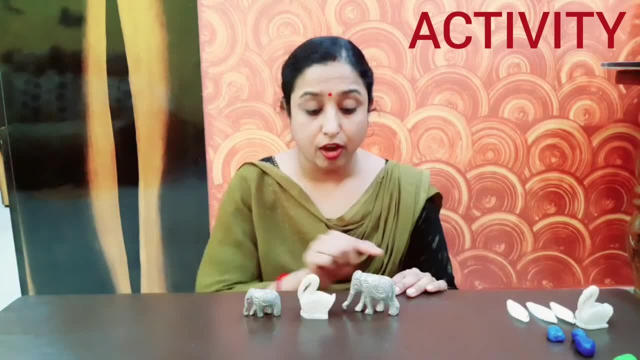 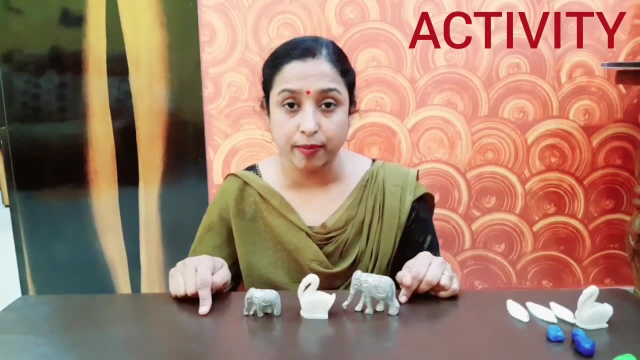 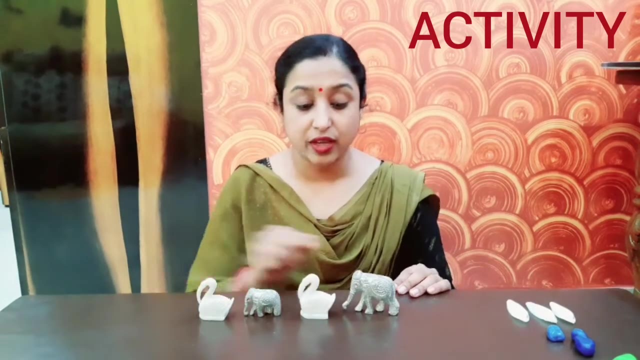 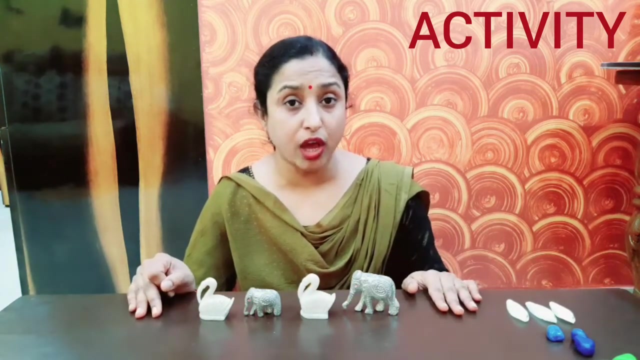 Then again elephant. Observe the pattern and recognize elephant, swan, elephant, Then what will come next? Yes, swan. So let's complete the pattern. So this is a pattern. So this is a complete pattern. In this pattern, a specific rule has been followed. 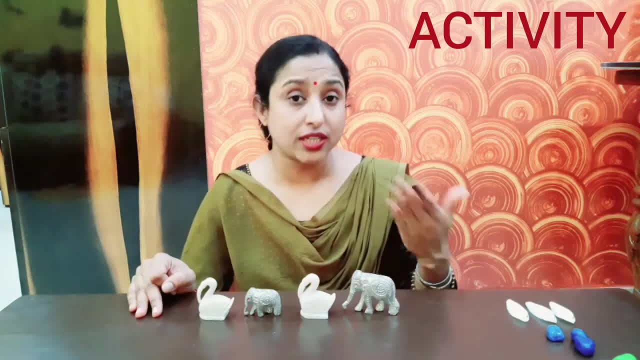 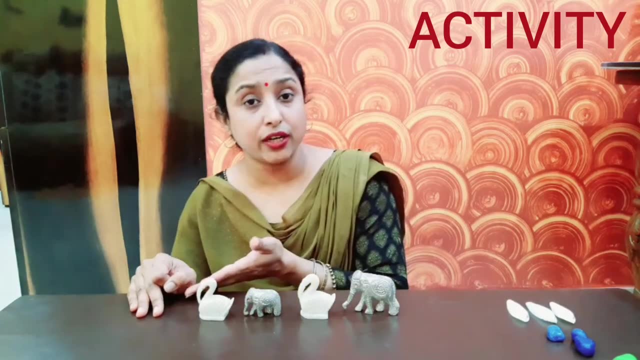 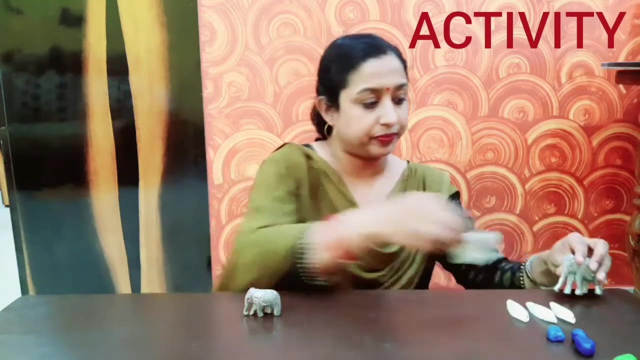 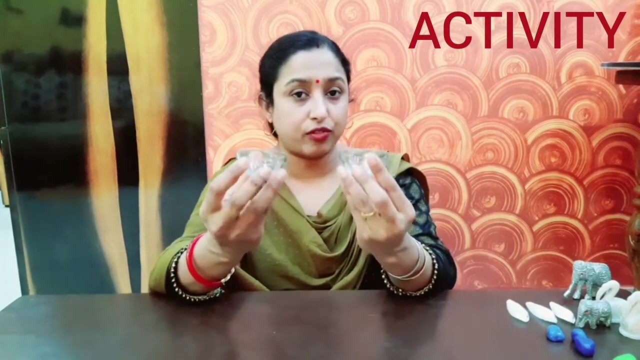 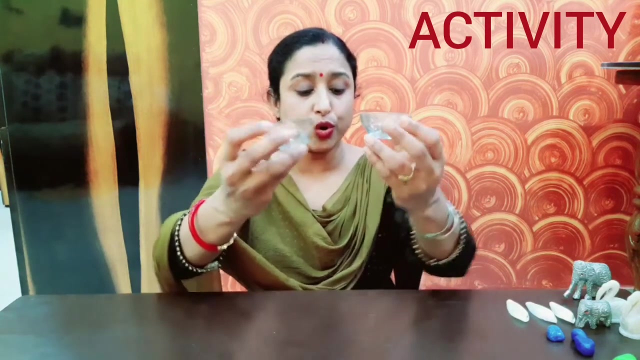 Here I've arranged this object alternative wise, one after another, Elephant swan, elephant swan. So now it's a complete pattern. Now we'll go over to the next example. So, children, Look at here. What are these? These are bowls. How many bowls are there? Two, One, two. 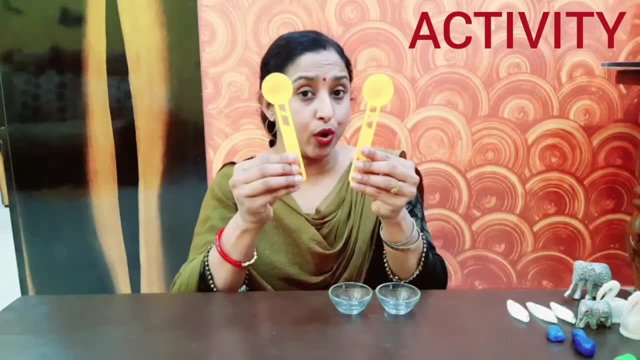 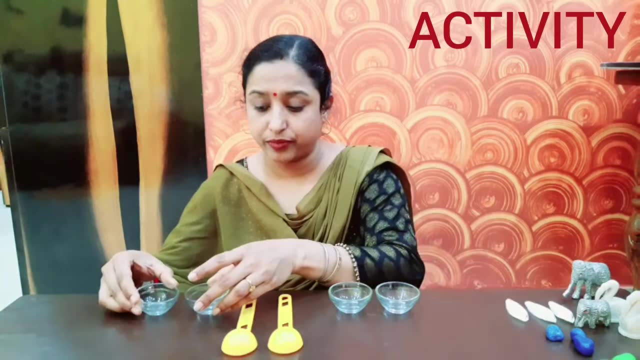 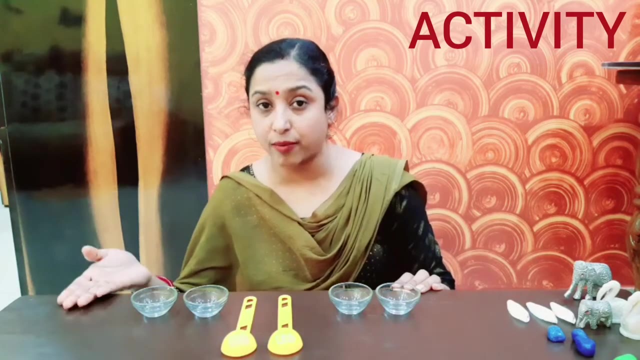 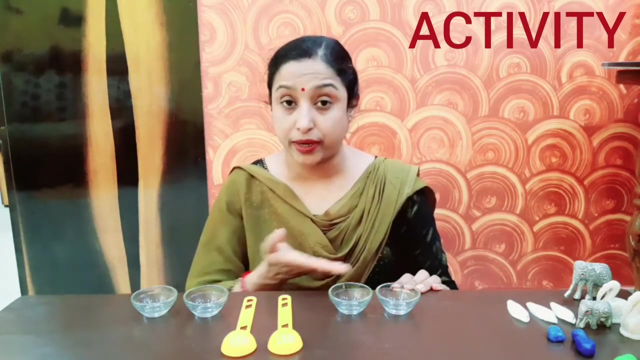 Then I have two spoons. Then again, I'm going to keep two bowls. Look at the pattern: Two bowls, two spoons, Two bowls. Then what will come next? Yes, two, Two spoons. So we have to keep two spoons over here to complete this pattern. 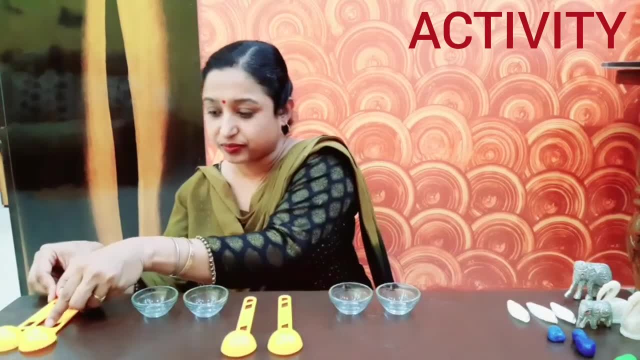 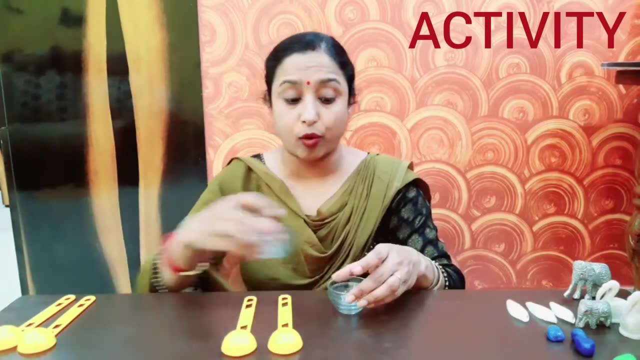 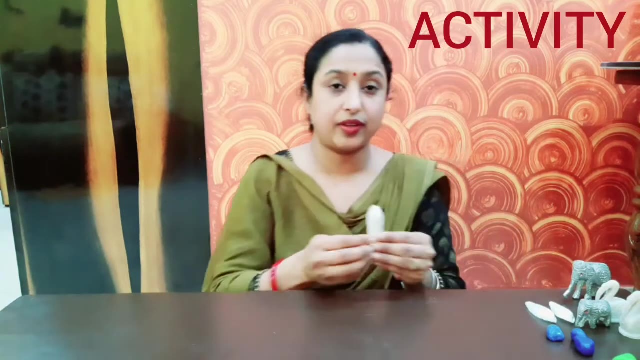 So let's complete the pattern. So it's a complete pattern. Next, again, I'm going to give one more example. So, children, please keep watching. This is a shell. Next, I'm going to keep a bowl. 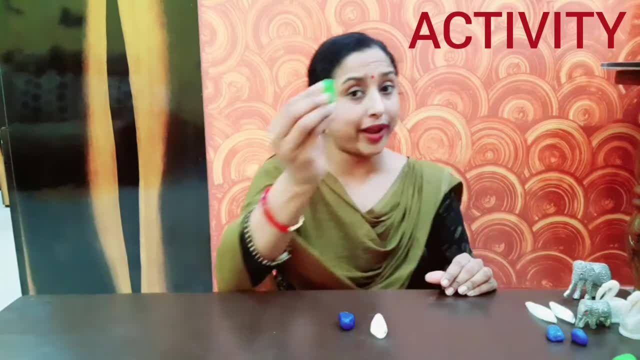 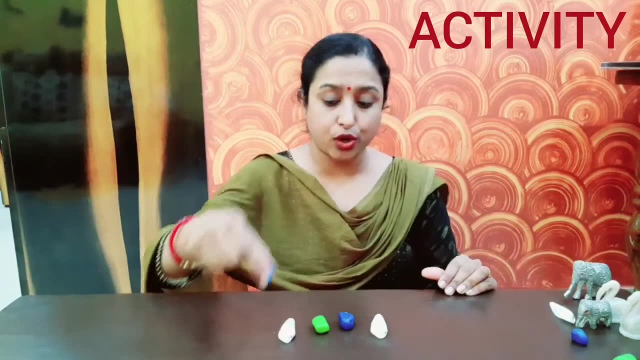 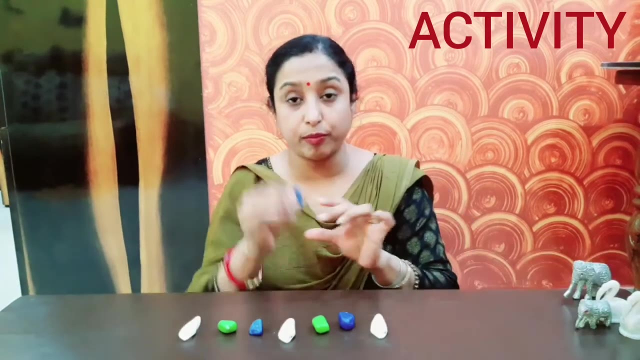 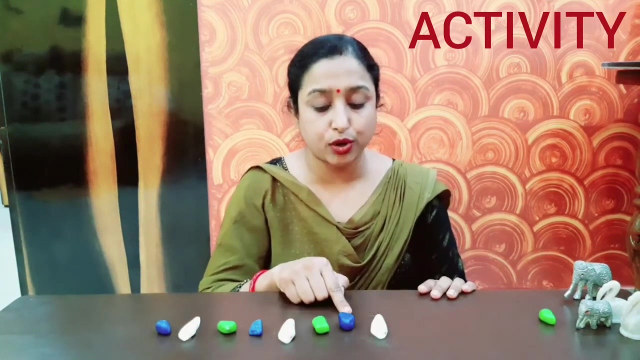 A blue stone, then a green stone, Again shell, blue stone, green stone, Again shell, then blue stone. Look very carefully: Shell, blue stone, green stone. Shell, blue stone, green stone, Shell, Blue stone. 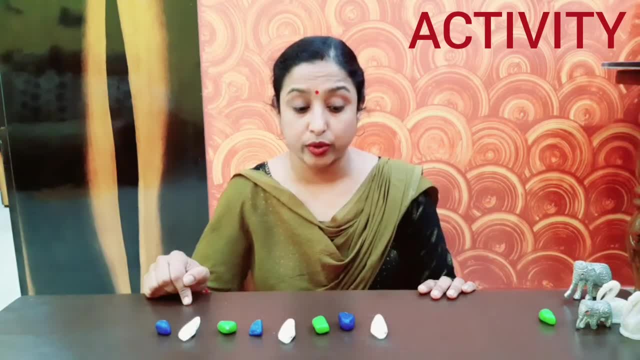 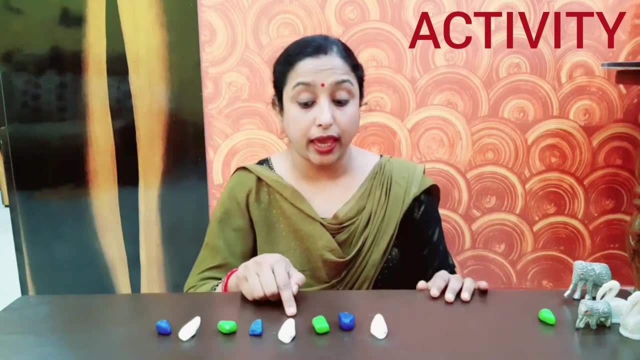 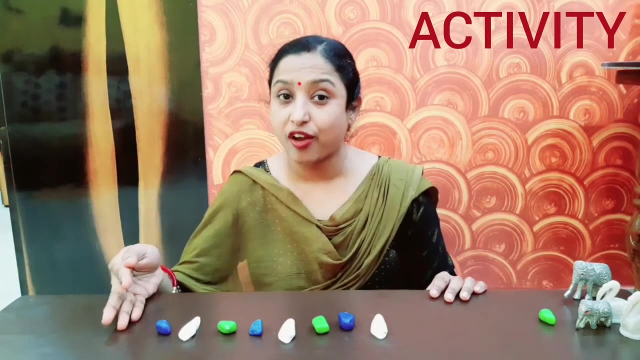 Is it a complete pattern? No A, B, C? Yes, you can assume in this way also: A B, C, A B. So what will come next? Obviously C. Here C means green stone. 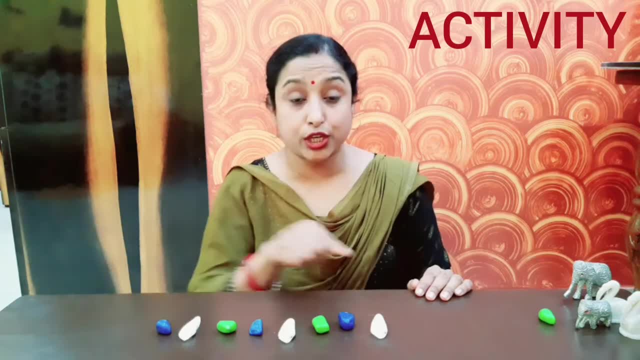 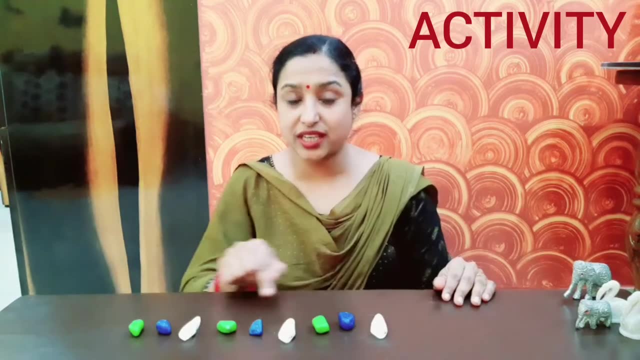 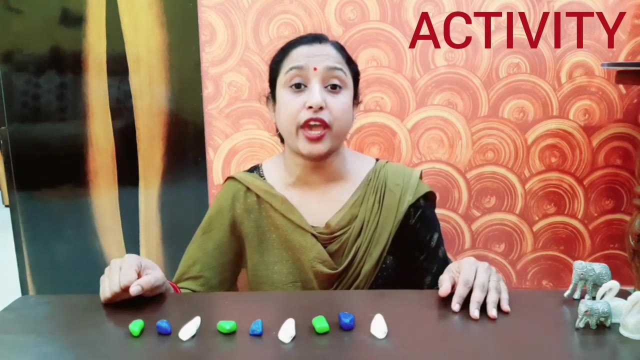 So we have to keep green stone over here to complete this pattern. So let's complete the pattern. Yes, Now this is a complete pattern. So, children, I think the concept of pattern is clear to everyone. You can also make different types of patterns by using different objects.